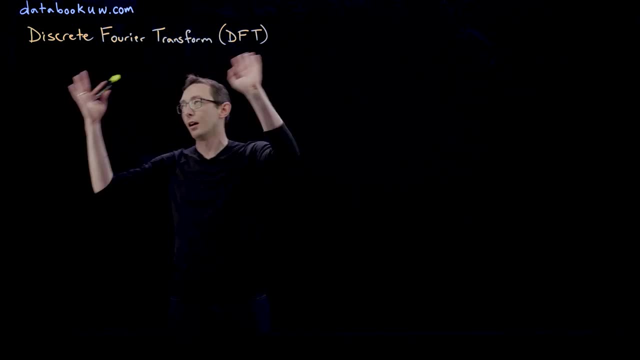 finite series and not the infinite Fourier transform integral, But through some joke of history it is now called the discrete Fourier transform or the DFT, And this is an extremely important concept, which will eventually lead to the fast Fourier transform, the FFT, which is probably the most powerful algorithm of the last century, maybe of all time. 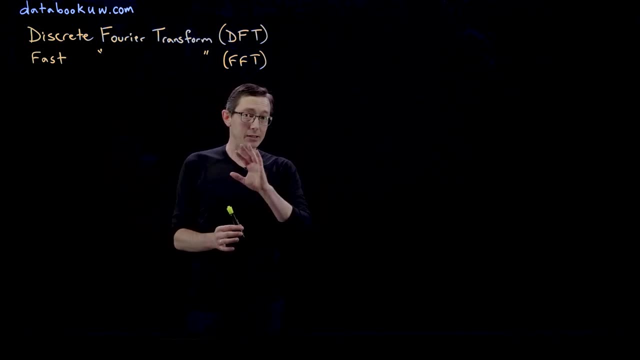 It's one of the most important algorithms today. It's used for image compression, audio compression, signal processing, high-performance scientific computing- you name it. Fast Fourier transform is probably at the heart of some of these computations, And what I want to get across right now is that the 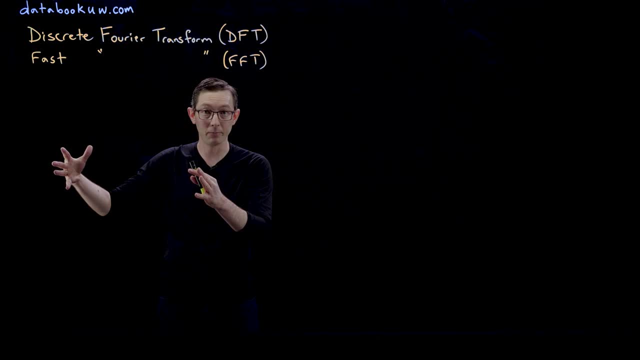 discrete Fourier transform is a mathematical transformation that can be written in terms of a big matrix multiplication. The fast fourier transform is a computationally efficient way of computing the DFT that scales to very, very large data sets, So in some sense these are kind of synonymous. The 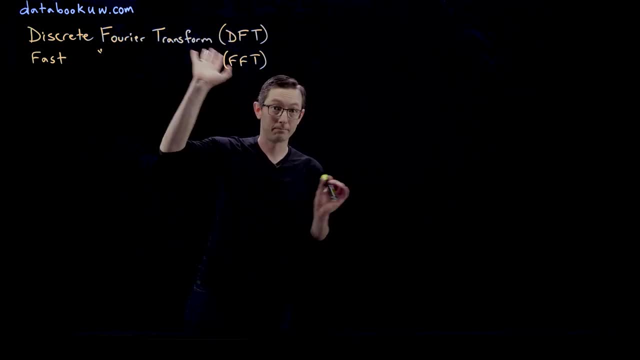 FFT is how we compute the DFT. Okay, I'm going to tell you about the DFT, the discrete Fourier transform, and soon I'll show you how to actually can Numerically implement this via the FFT. okay, so we talked about approximating. 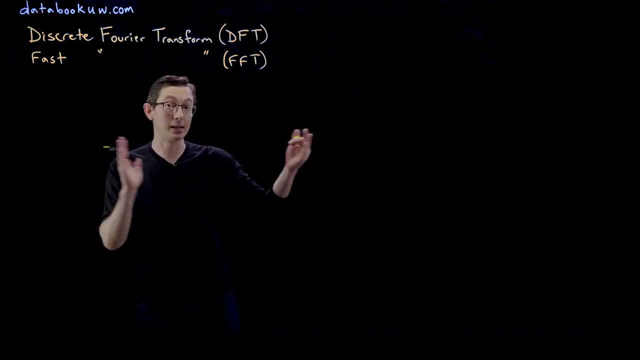 Functions that are periodic, using infinite sums of sines and cosines, and we show that this is this is possible, But in many, many cases, most of the time, I don't have an analytic function. I have measurement data from an experiment or from a simulation. Okay, so what I? what I often have is some F defined at discrete locations. 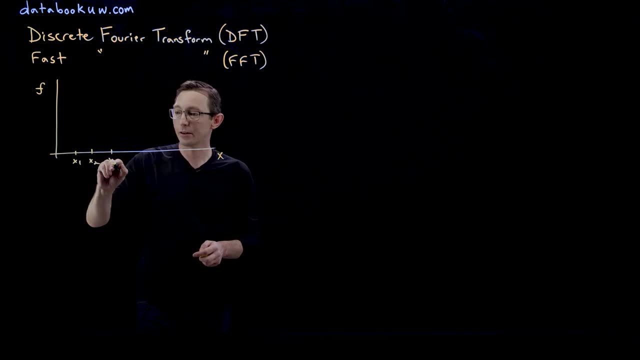 x1, X2, x3, all the way up to some X, and so I have a discrete vector of data, Some function, and maybe we believe that there's a continuous function underlying this data, But I'm only sampling it at these discrete locations: X1, X2, X3. 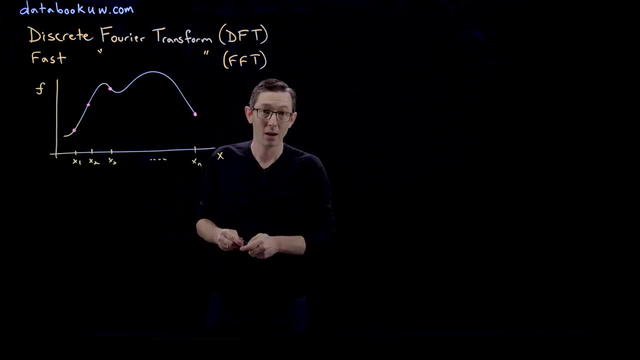 And so on and so forth, up to X, n. okay, so what I have is a vector of data. In fact, I'm just going to literally write this out: I have a vector of data f1, f2, f3, Dot-dot-dot-dot-dot all the way down to F, and 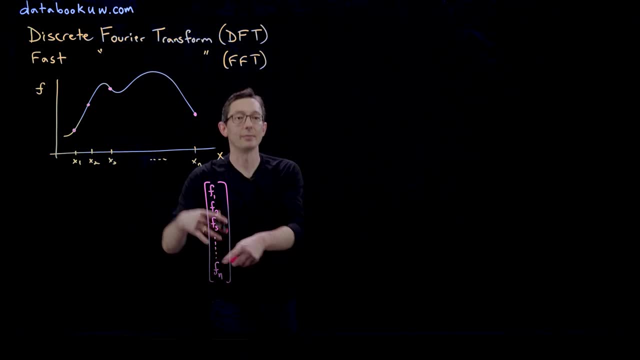 Okay, this is going to be my- I'm just going to call this- You know some vector of data and what I'm going to want to do is Fourier, transform, compute the discrete Fourier series Of that data Vector. okay, So I also want to break this data up into a sum of sines and cosine, and this can be very useful. 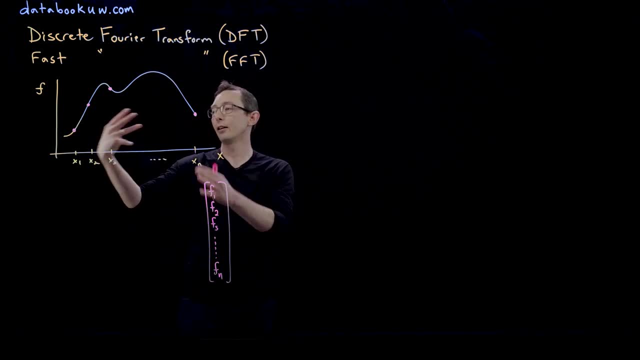 You can figure out if this is audio data. You can figure out what are kind of the, the tones that add up to make that audio data. I always tell my students: You know, what I want to do is build an iPhone app so you put it on the roof of your 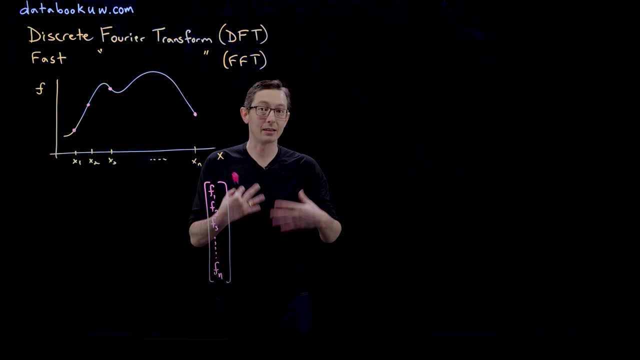 car or the the hood of your car, and it listens to the audio signal. it computes a Fourier transform and, based on the frequency content, Maybe it can diagnose if something's wrong with your car, like you have a belt slipping or some kind of vibration that shouldn't be there. 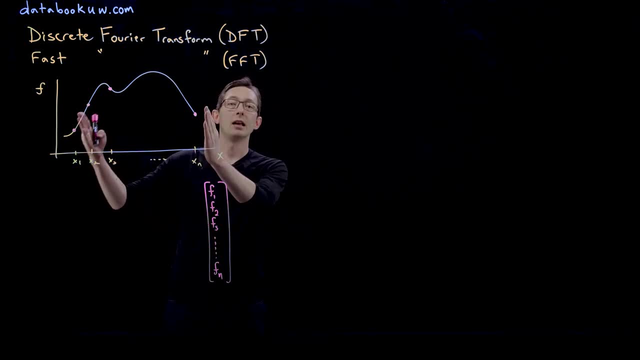 Okay so. so turning a data vector Into its sine and cosine components through this discrete Fourier transform can be very, very useful. It's also Nice to compute derivatives, to approximate derivatives of data Using using these Fourier transform derivative properties. okay, so I'm gonna walk you through. 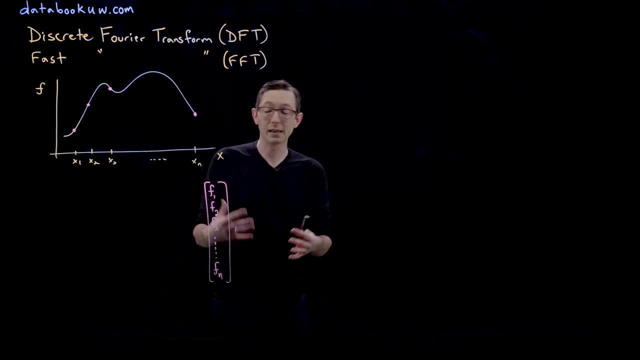 What the Fourier transform, the discrete Fourier transform, is how you can write it as a big matrix multiplication, But remember, it's basically just a Fourier series on data instead of on continued on Functions, analytic functions. okay, so let's just get started. So I'm just gonna write down what the the Fourier. 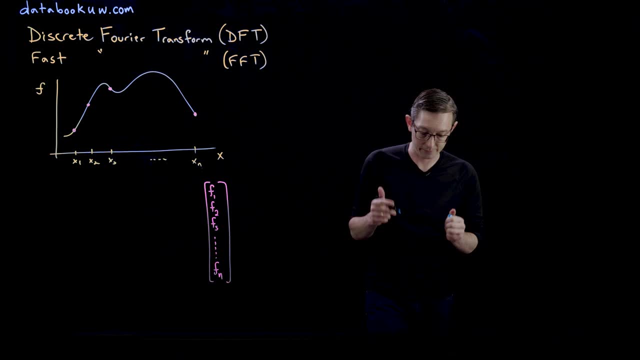 Discrete Fourier transform is, and then I'm going to show you some ways of interpreting this. okay, so for each of these data points, fk, What we're going to be able to do is compute a. As you might imagine, what we're going to try to get out of this is some vector of Fourier coefficients, f1 hat. 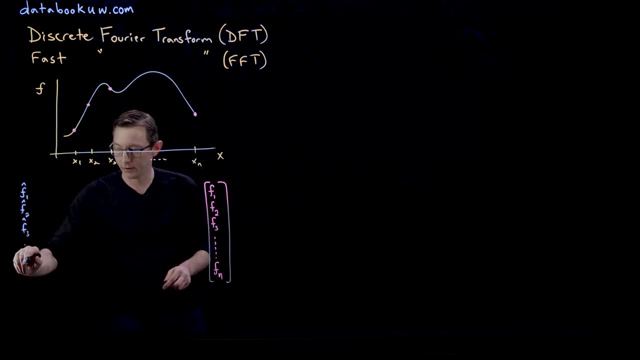 f2, hat, f3, hat, all the way down to f and hat. So, just like we took our function f and we turned it into these coefficients that multiplied our cosine and sines, That's what we're doing here. We're taking our data f and we're going to obtain this Fourier transform. 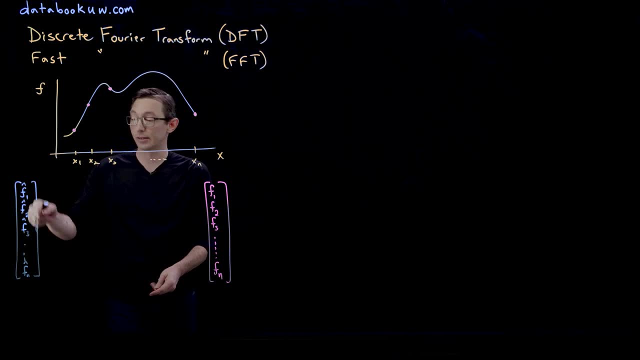 vector f hat of frequency components. So f1 hat will tell me how much of that first low frequency is in the data. f2 hat will tell me how much of that next higher frequency is in the data, and so on and so forth. where f n hat is. 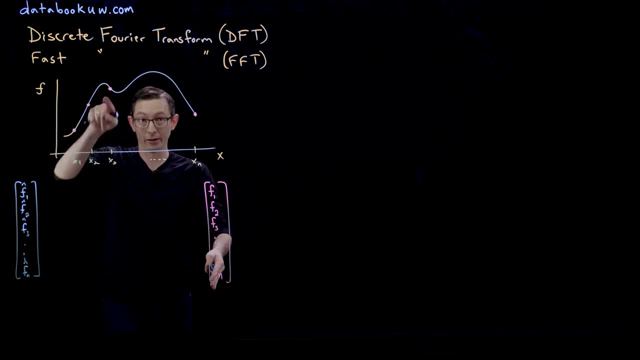 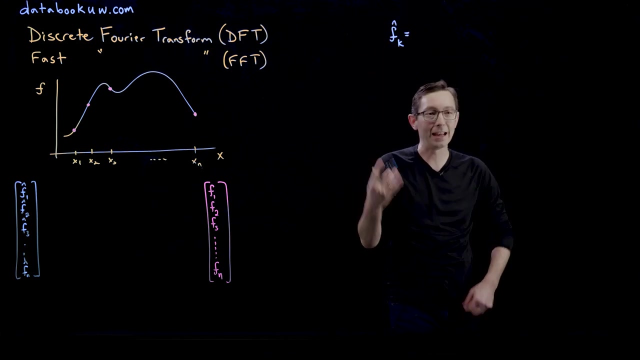 The highest frequency possible with n data points if it was going, you know, as fast as possible oscillating over n data points. And so the way that we get that f hat vector, we say that f hat k, Maybe I'll write it up here: f hat k. the kth Fourier coefficient is: 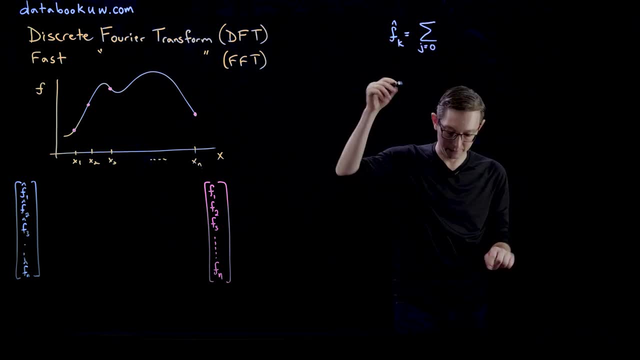 a sum over all of my, all of my data, to n, minus 1 of My data f, j, the jth element of my data times, e, to the minus i, 2, pi, j, k Over n. this is kind of a pain. I'll walk you through all of these terms here, Okay so. 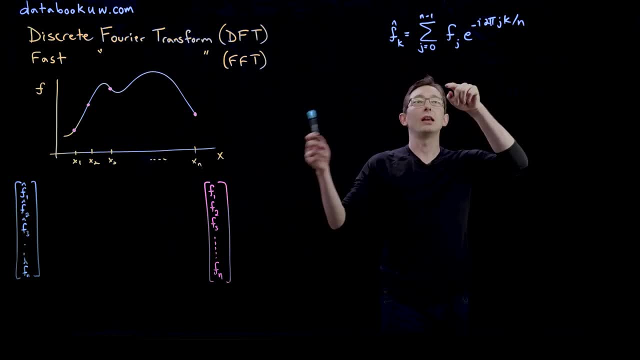 the kth Fourier coefficient is Obtained by taking the sum over all J data points at the jth frequency times, the kth frequency Divided by n. and I'll tell you what this kind of e to the i, 2, pi, j, k over n means in a minute. 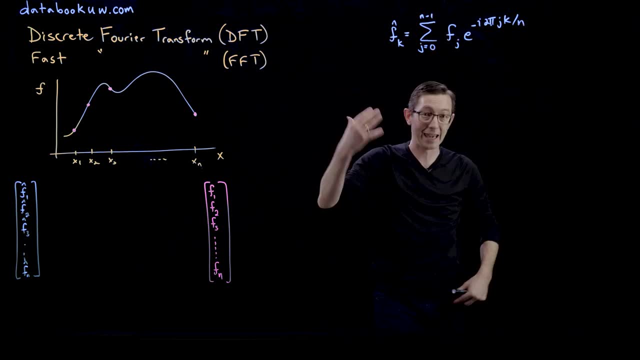 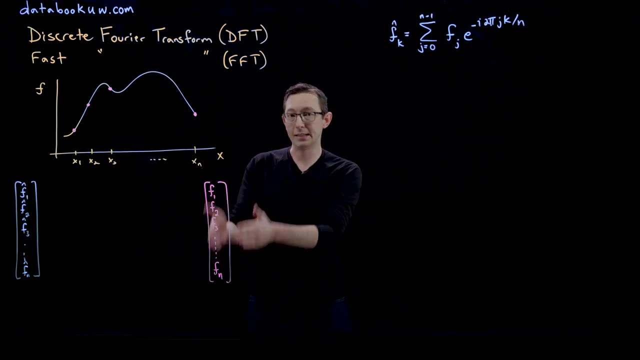 Okay, but this is how you compute all of those kth Fourier coefficients and similarly, just like in a Fourier transform or a Fourier series. if I have my data, I can get my Fourier transform, But if I have my Fourier transform, I should be able to go back and reconstruct my data. 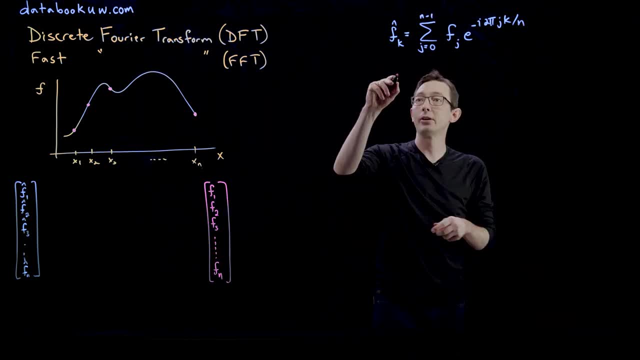 And so I'll write down what that is. and it's again. It's pretty similar. so f? k- once I had all of these blue hats, the f? k is again a sum over all frequencies now, of J equals 0 to n minus 1 of my f. 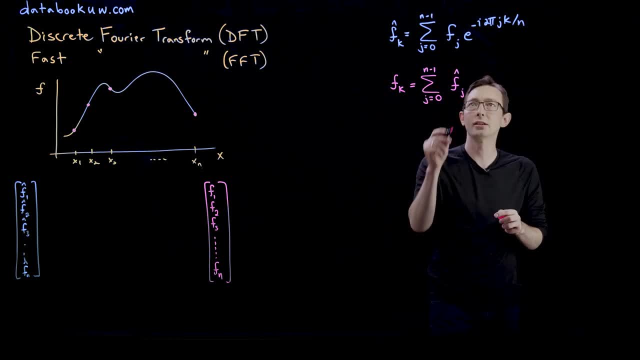 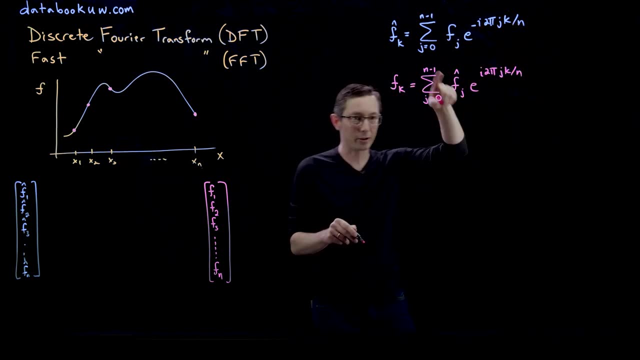 J hat, okay, my jth Fourier coefficient times. now: e to the positive, i, 2, pi, j, k, J, k over n. so this is very, very similar to the Fourier transform pair, Where this is a negative exponent and this is a positive exponent and this whole thing is. 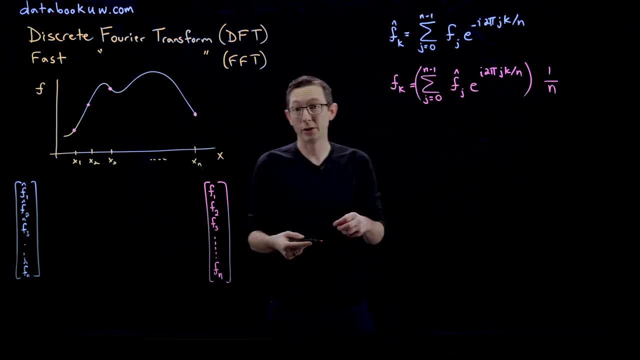 times 1 over n. Remember, just like in the Fourier transform, this had a 1 over, I think, pi or 2 pi. this also has two slightly different normalization. Okay, and so what this means is that if I have, if I had my data, kind of f1. 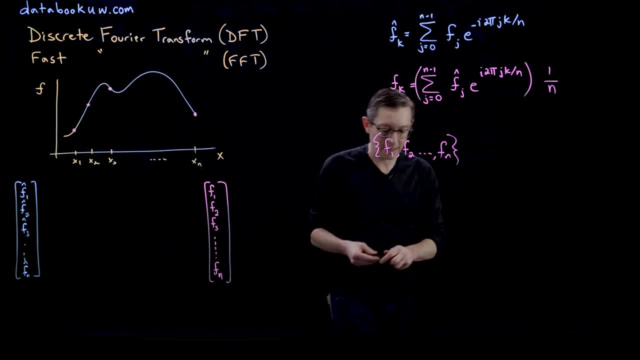 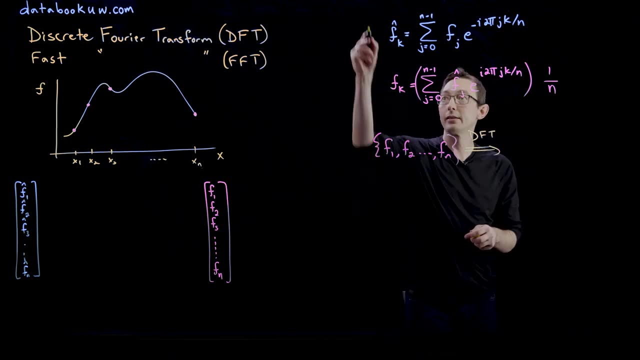 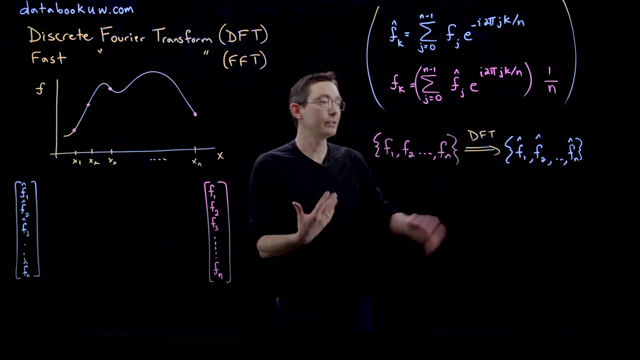 f2, dot, dot, dot to f? n. I Can run it through this Fourier transform, this DFT, this discrete Fourier transform Here. this is my DFT And I can get my Fourier frequencies: f1, hat, f2, hat, dot, dot, dot, f and Hat. okay, and these literally are the f1, f2, f and hats are literally telling me how much. 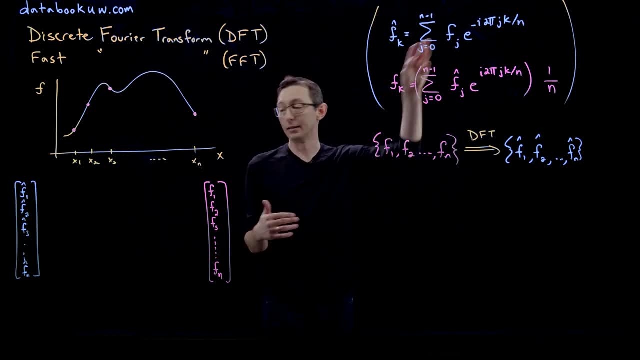 Of each, each frequency I need to add up, to reconstruct this data in F, okay, And there will be some subtleties I'll tell you about, But to compute this thing. this is kind of interesting is that notice that all of these, These, these terms in the series are: 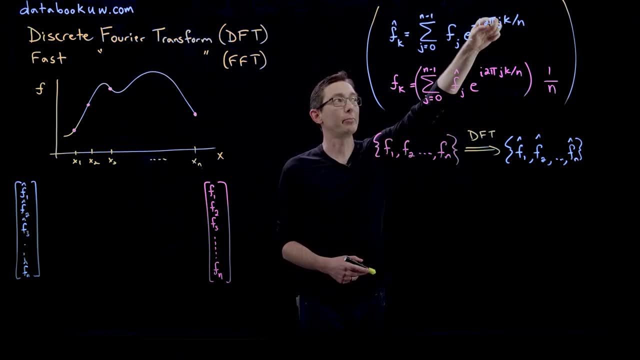 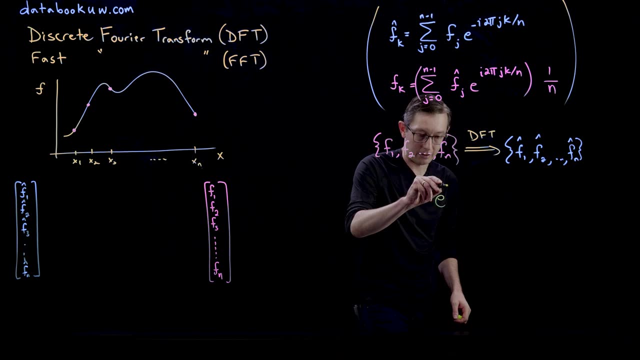 Multiplying these exponentials, which are some integer multiple of e to the i, 2 pi over n. okay, So we have this kind of e to the minus 2 pi i Over n. I is the, the complex of the imaginary variable I, square root of 1.. I'll just write: I equals. 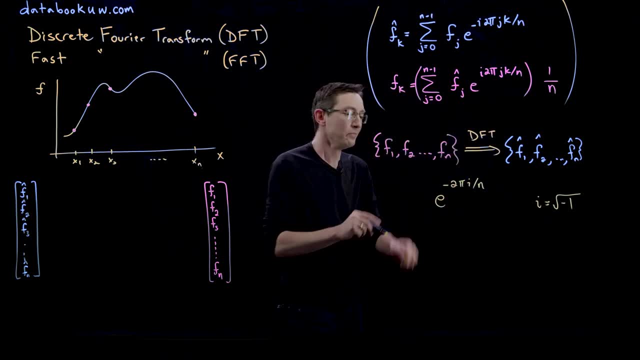 square root of negative 1. okay, this is I, and This defines a fundamental frequency. this defines some omega n. Okay, which is some fundamental frequency that is related to To what kinds of sines and cosines I can approximate with n discrete values in a domain x. okay, 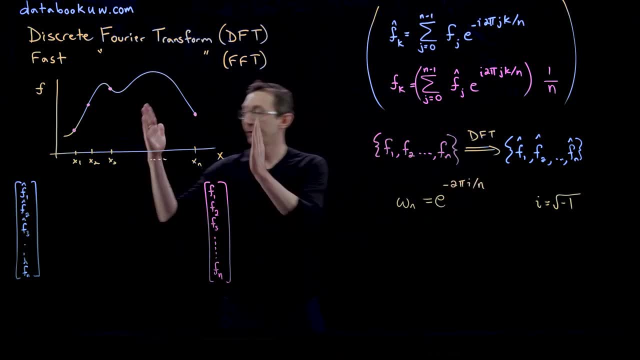 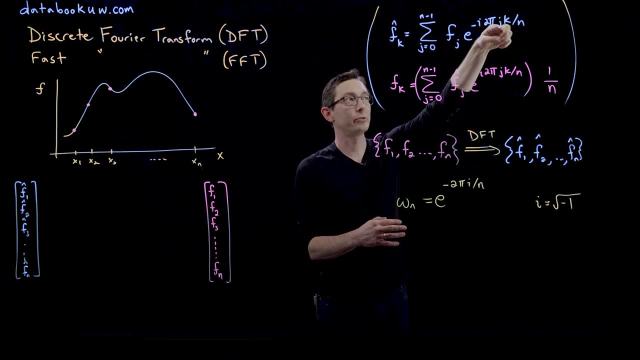 So this is kind of the fundamental frequency we get to work with. if I have an interval with n data points and All of these Fourier transforms are adding up integer multiples of that fundamental frequency times my data, and the same thing with my inverse Fourier transform. okay, so we're going to be able to use this fundamental frequency, Omega n, to compute a. 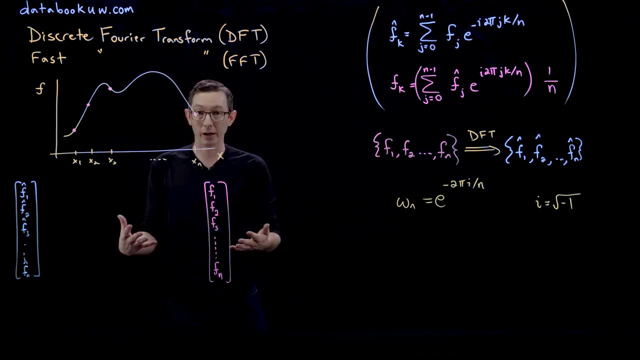 Matrix that would multiply my data and give me my Fourier transform. so that's really, really important and I'm going to write this out here, Okay, Okay, good, so, So we have this: this sum over the data to compute the Fourier transform and the inverse Fourier transform. 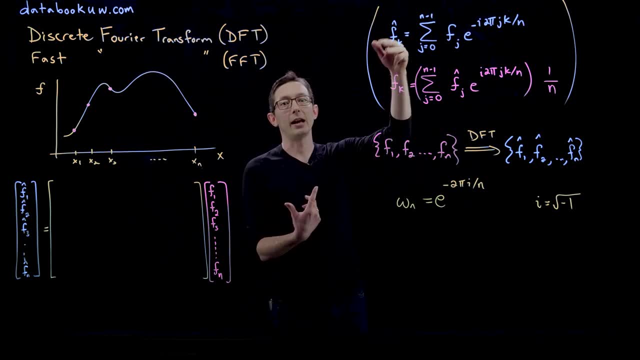 But I don't want to go, you know, for k 1, for k 2, for k 3, for k 4, and compute this whole sum. This seems very tedious. This would be kind of two big for loops if I want to do this loops if I wanted to actually code that up, and I don't want to do that. So instead, what we're going, 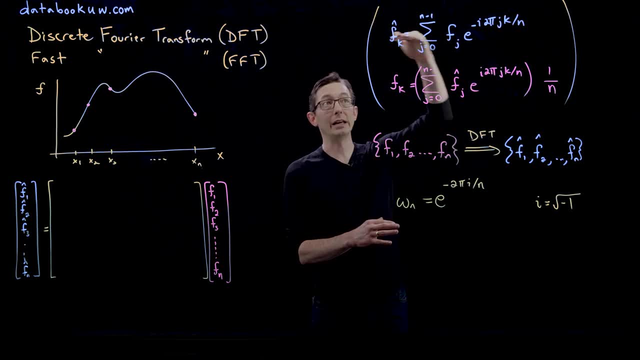 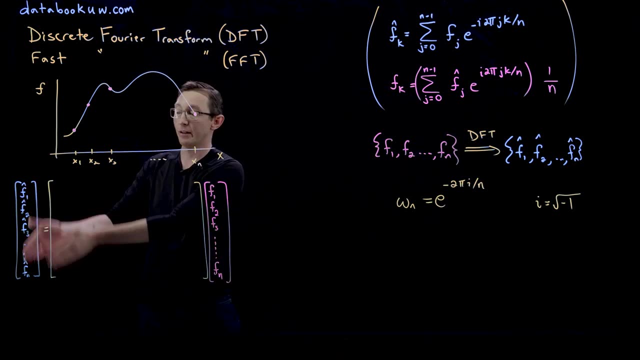 to do is we're going to try to write what this sum would be for each of these k's in terms of a matrix operation, where I take my data vector and I multiply it by a matrix to get my Fourier transform vector, And I'm going to write it in terms of these fundamental frequencies, omega n's. 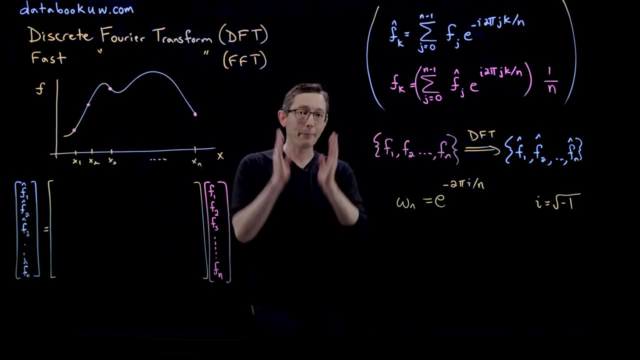 okay And I'll point out: you can absolutely go back to your definition of the Fourier series, the complex Fourier series, where you had it written in terms of the complex exponential, and you can show that this is exactly what you would get if you took your Fourier series and 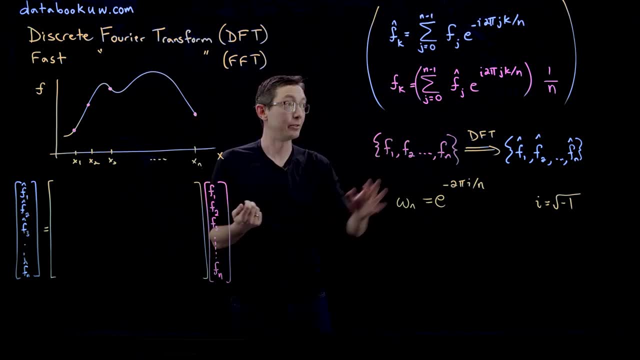 approximated it with n discrete values in the middle. This is exactly analogous to the cosines and sines of those discrete frequencies in the Fourier series. Okay, good, So we have this fundamental frequency and we're going to walk through, and sometimes what I like to do is just 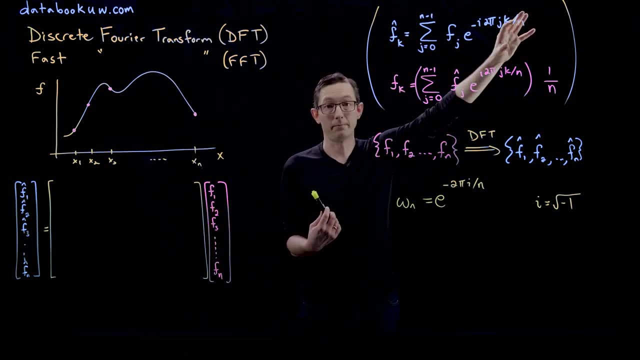 think, if k was 1, what would this series look like? Okay, so if k was 1, I would take all of my fj's and multiply them by some- the first row vector- and that would tell me the coefficient on each of those fj's. 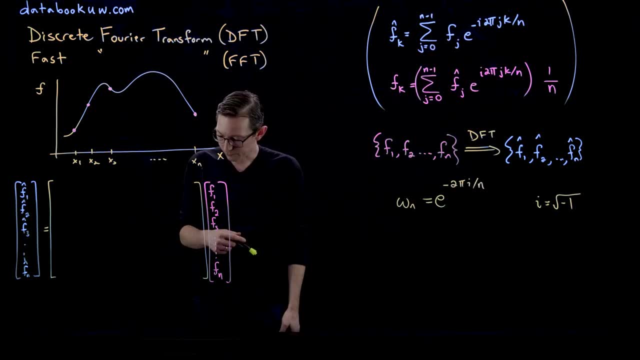 okay. Now if k was, yeah, I probably should have k0.. Yeah, sorry, I'm being pretty sloppy here. Let's say that I actually have a zeroth index here. Let's say I have an x0, and that this is. 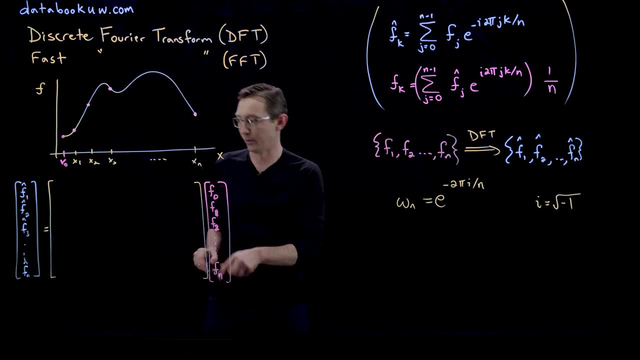 f0,, f1,, f2, all the way up to fn. and this is f0,, f1, f2, all the way up to fn. This will make a lot more sense if j my data has to be indexed from 0 to n-1, okay. 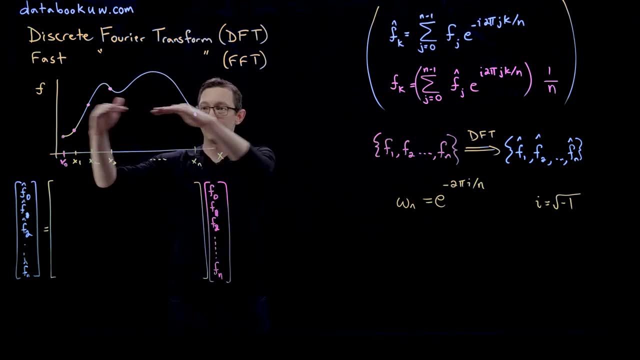 So the zeroth, this is the zeroth frequency kind of the constant value. If I had k equals 0 here, then all of my exponents would be e to the i times 0, because k is 0. And either the 0 is 1.. No matter what j is, if k is 0, this whole exponent is 1.. 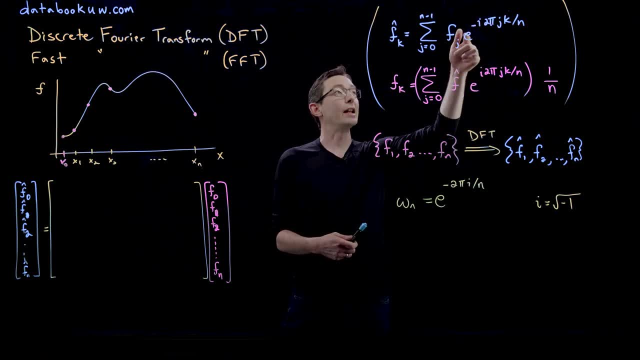 Is, uh is. this whole exponent is 0.. So either the 0 is 1., And so the coefficient on every single data point here is 1, and I'm adding up f0, plus f1, plus f2, plus f3, all the way to fn. 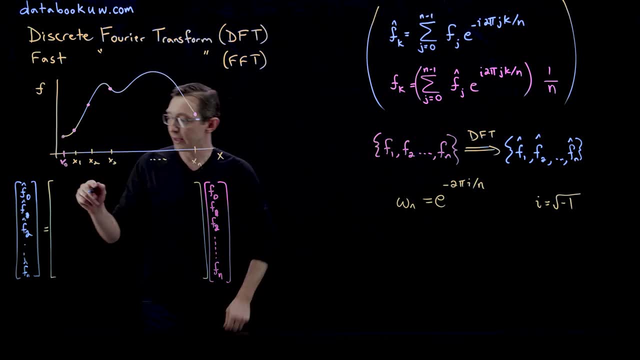 will give me the first, the 0th F hat. so this row is 1. maybe I'll make it in yellow. this is is 1, 1, 1, dot, dot, dot 1. okay, this entire first row is just ones. now for the second row. now let's figure out what happens for F 1 hat. okay, so in 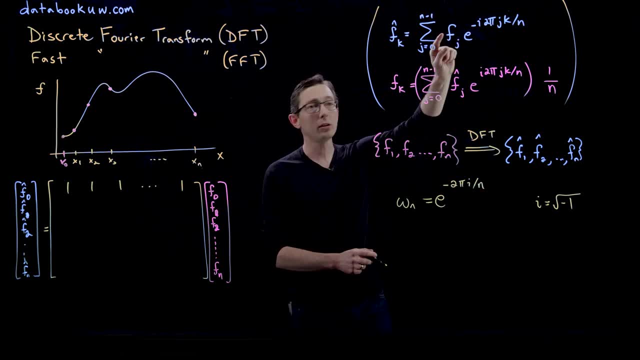 K equals 1. now all of these coefficients multiplying my data: F for J equals 0, I get e to the 0 is 1. okay, for J equals 1, I get e to the minus 2 pi I divided by n, remember K is 1, so that's just Omega. when J equals 2, I get: 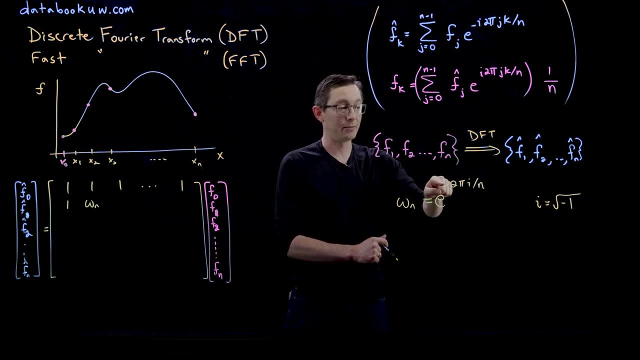 basically Omega. squared, I get e to the minus 2 pi. I times 2 divided by n. this is Omega. and squared, dot, dot, dot and eventually, at the very end, I'll have Omega. and to the power n minus 1, okay, and I can keep going down. if K was 2, then I would have. 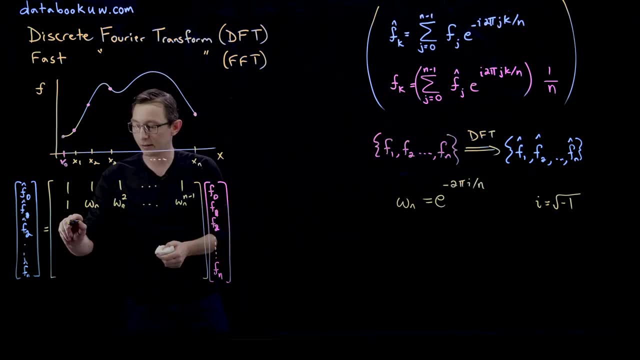 everything you know. multiplying 2 in the exponent. so I would still have, for J equals 0 a 1. here I would have an Omega n squared because my K is 2. I'd have Omega n to the fourth, dot, dot, dot. Omega n to the 2 n minus 1, and so on and so forth. you can. 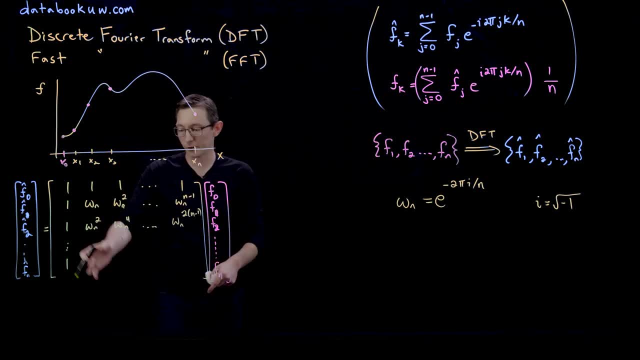 just go down the list. I'll always have ones on the first row and the first column down. here I'm gonna have something like Omega n to the n minus 1, Omega n to the 2 n minus 1, dot, dot, dot and eventually this last entry is going to be Omega n to the n minus 1 squared. 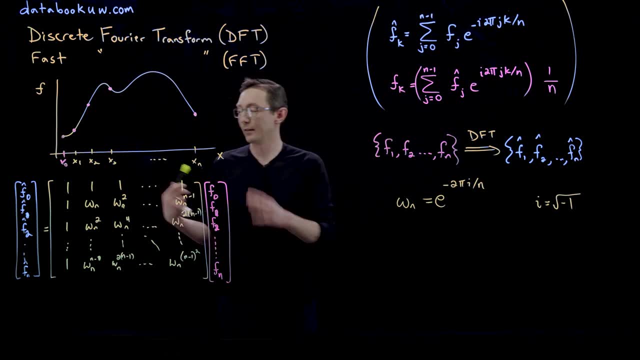 okay, so this is something you can. you can readily kind of convince yourself that every row of this is one value of K here, and you can figure out what the coefficients are of the data that will be the row of this, this matrix DFT here. okay, so long story short what I'm trying to. 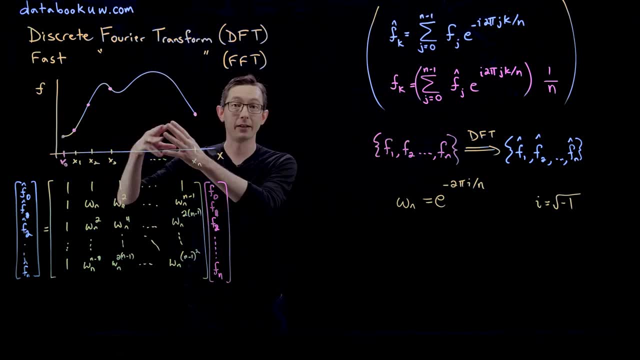 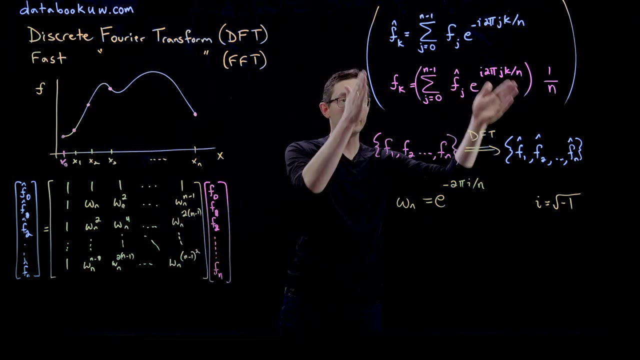 convince you of is that if you have a data vector instead of a, an analytic function, so you just have data in these, these pink dots here, you can still compute something like a Fourier series, like a Fourier transform, but it's the discrete Fourier transform, okay, and the form of the: the discrete Fourier. 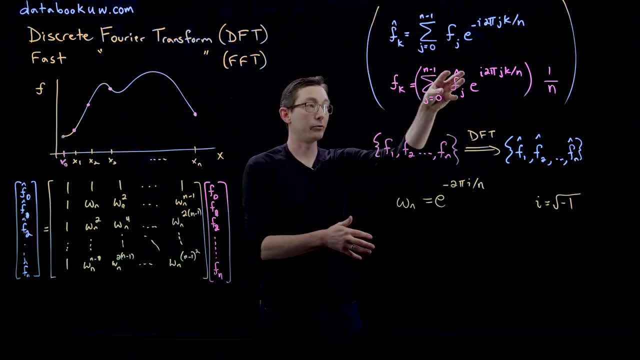 transform pair to go from data to Fourier coefficients or to go from Fourier coefficients back to your data. looks very much like a Fourier series, but because this is defined on discrete data, I can write it as a big matrix operation. okay, so this here is the DFT matrix. this is the DFT, the discrete Fourier transform matrix. and if 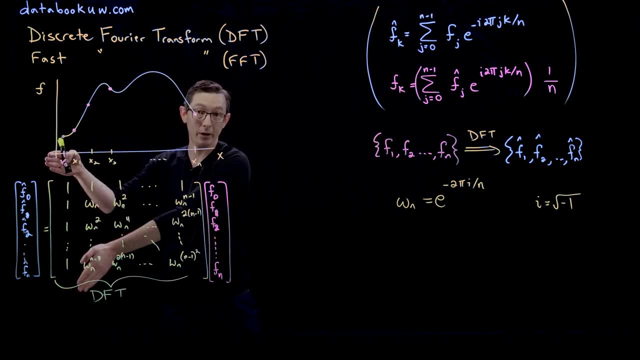 you had your, your vector of data. you multiply it by this matrix, you get your Fourier transform out very, very useful. okay, and these Fourier coefficients. you'll notice that this is a complex number. okay, this is e to the. this has a cosine plus an I sine part. this is a complex number, so this is a complex. 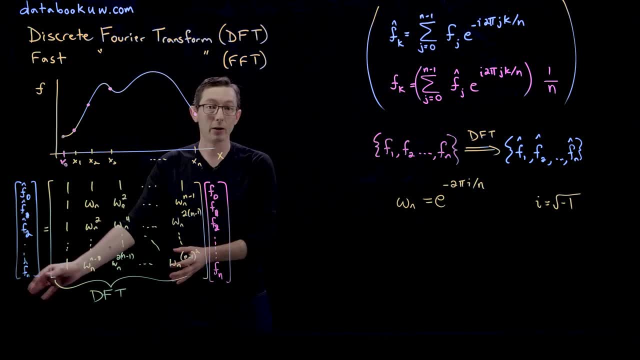 matrix and these Fourier coefficients, these blue Fourier coefficients are complex valued, and so these somehow tell you how much of that zeroth mode, cosine and sine mode there are, but it also tells you the phase. okay, so the magnitude of this complex number tells you how much magnitude of that. first, 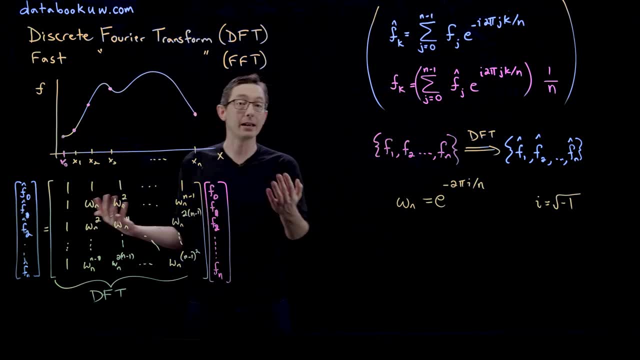 mode you have. and then the cut, the, the phase angle of that complex number tells you you know how much cosine or how much sine or what phase in between your, your sine and cosine is okay. so every single one of these values is a complex number and the 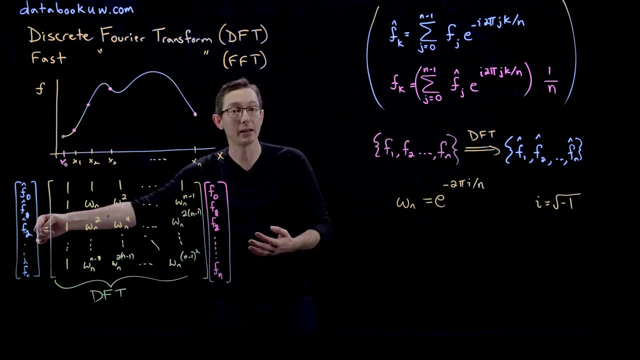 magnitude tells you how much of that set, that that second frequency sine and cosine you have, and the phase tells you what is the the phase between cosine and sine and it gives you exactly the sines and cosines you need to add up to approximate your data perfectly. 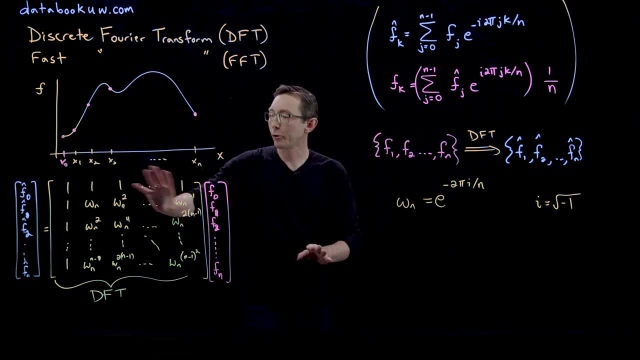 ok, so this is the discrete Fourier transform. this is pretty expensive to actually compute this matrix and multiply your data to up to compute this Fourier transform, and so what I'm going to show you in the next few lectures is how you compute this efficiently using the fast Fourier transform, so you never 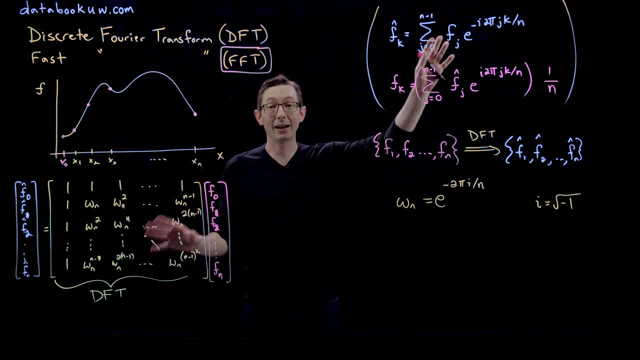 actually have to build this matrix and do this multiplication. this is how it's mathematically defined, but computationally we're always going to compute the DFT using the fast Fourier transform algorithm. ok, that's all coming up soon, thank you. 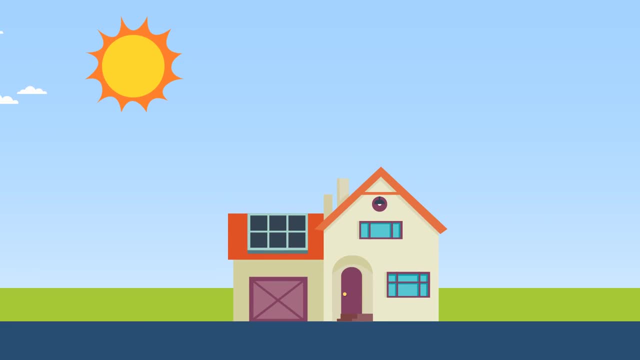 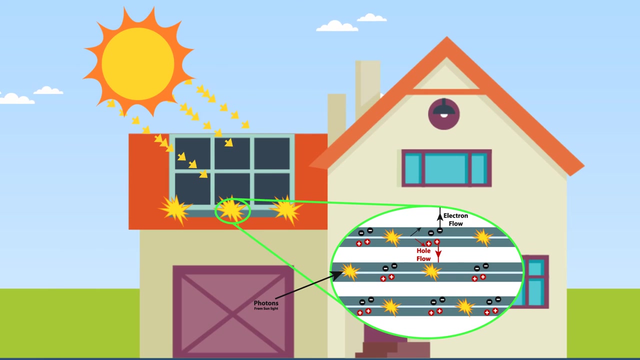 How solar power works. Solar power works by taking the energy from the sun's rays and converting it into electricity. The sun's rays contain photons. When these photons hit a solar module, electrons inside of the solar module move and an electrical current is created. This electricity then travels from the solar array to an inverter. 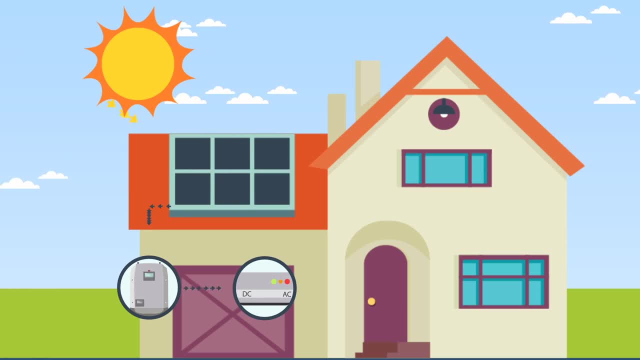 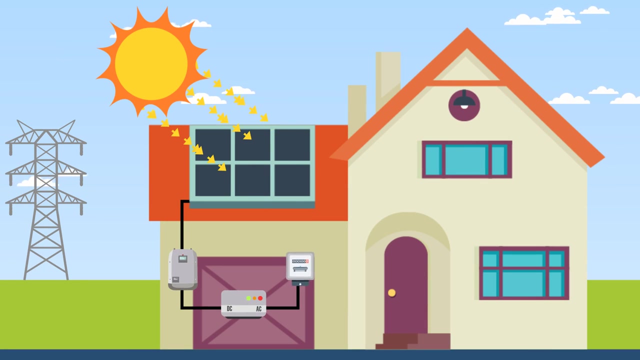 The inverter takes the electricity which is in DC or direct current form and switches it to AC or alternating current power. Once that switch is made to AC, the electricity is ready for household use. From the inverter the power is fed directly into the building's main electrical panel and can provide power to the site. 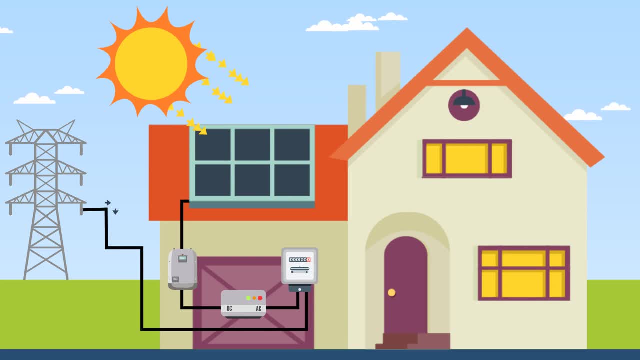 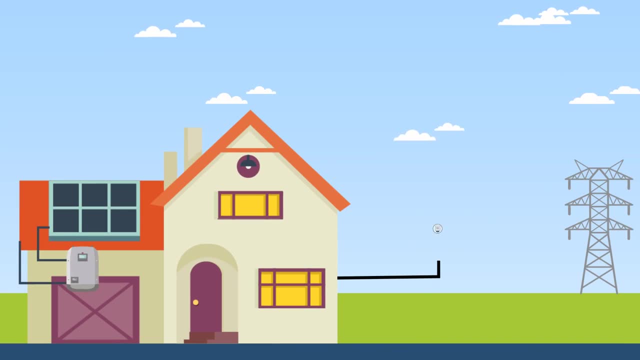 If the site demands more power than what is provided by the solar, it will pull from the utility grid. If the sun produces more than the site needs, Then that overproduction is put back into the grid for a credit in a process known as net metering. 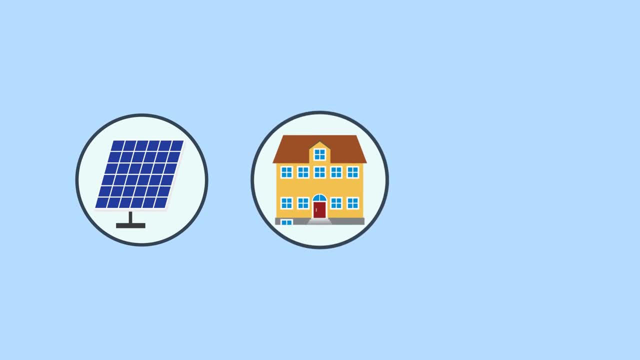 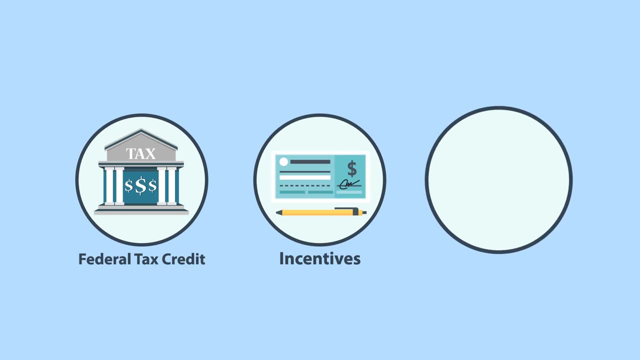 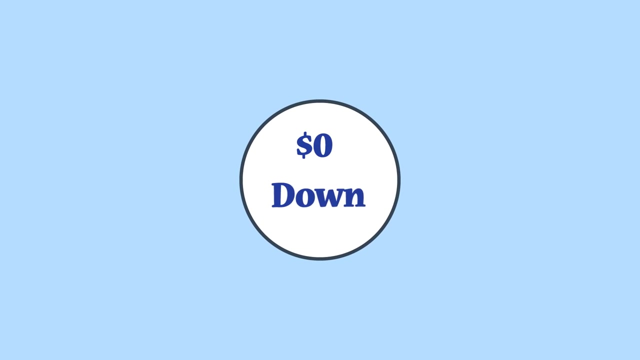 Today, solar panels will be viable energy producers on your home for over 20 years. There is a federal tax credit available and also incentives available at the state level which help to make the technology more affordable than ever. There are even no money down solar programs available. Contact Green Power Energy today for a custom solar quote for your home.